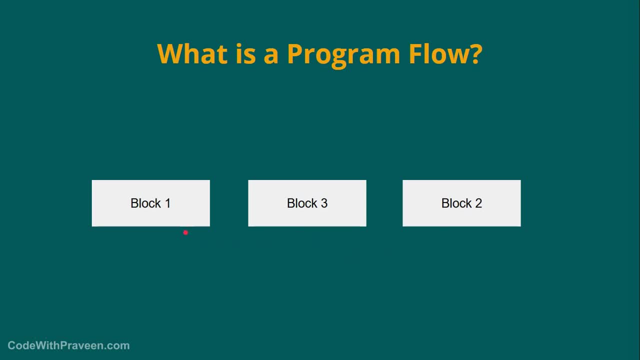 So this refers is as the program flow. So you have to tell the compiler or interpreter that you have to execute 1 first, then 2, then 3.. Now, if you compare this version now, here you have clearly defined that block 1 is the first, followed by the block 2 and followed by the block 3.. 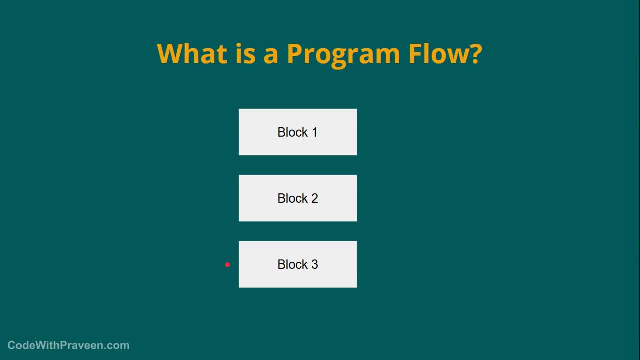 Now here it's very clear for the compiler or interpreter to know that this is a set of sequence of instruction it has to follow, And that block 1 has to be executed once, and then 2 and then 3.. Note that there are no conditions or no repetitions. 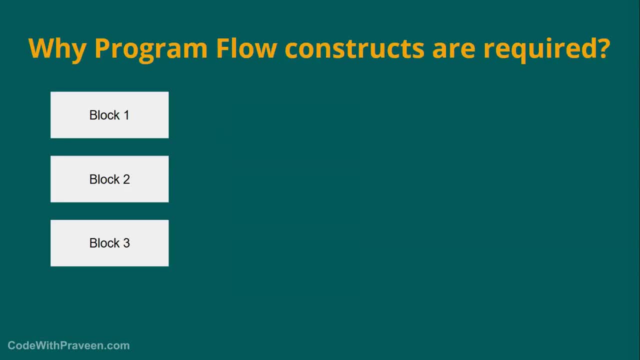 Just a simple set of program flow. Now let us consider why the different types of program flow are used. As I mentioned before, this is a simple flow. We have block 1, 2 and 3.. Now consider this example where you want to execute this block 2 only on certain condition. 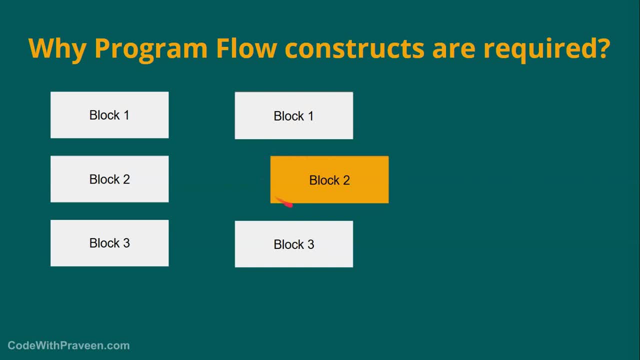 Meaning that if only certain condition is succeeded, then you want to execute this block 2. Otherwise the program has to execute only the block 3. How do you control this Without these program flow constructs? then these kind of set of conditional statements are not possible. 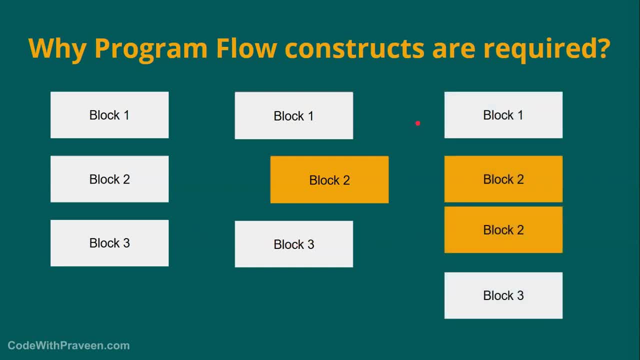 Now let's check one more condition Like, say, we have the block 1 and you want to execute this block 2 n number of times. Say, in this case, you want to execute this couple of times and then followed by the block 3.. 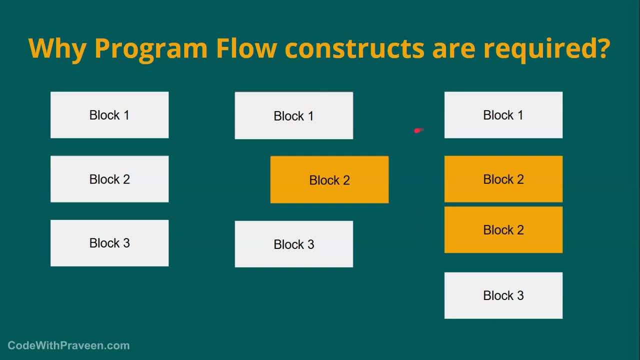 So when the actual program executes, it follows like block 1, then the block 2, then the block 2 executes again and then the block 3.. Now how do you tell it to execute this block 2, say 2 times in this case? 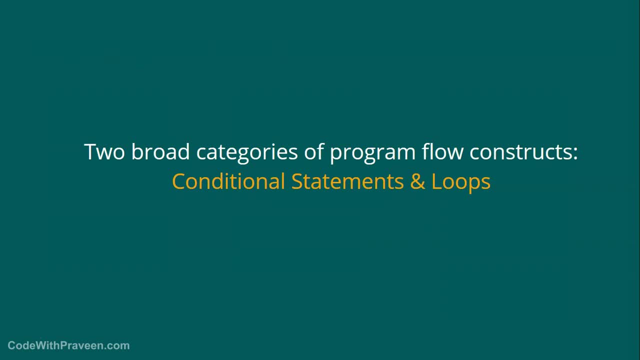 Now coming to the programming or the coding aspect, how do you define this set of program flow constructs In any typical program? you can define a set of program flow constructs In any typical programming language. we have two broad categories. They are namely conditional statements and loops. 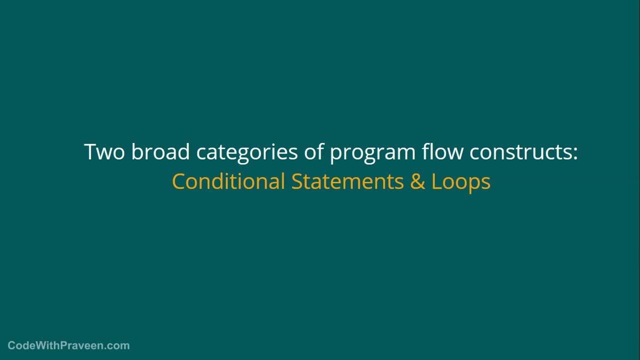 In the next few set of videos we will go deeper on these two topics. In the next video, let's see what are the first type, which is referred as the conditional statements. In this video, let us see what are conditional statements. 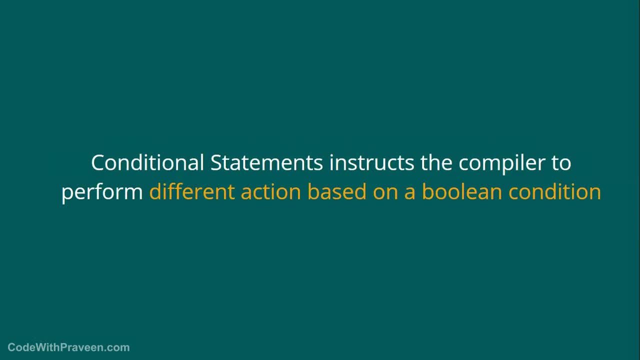 Conditional statements instructs the compiler to perform different action based on a Boolean condition. In the previous video we saw that the program flow constructs refers to how do you tell the compiler or the interpreter to execute specific set of instructions? These conditional statements are used to tell the compiler. 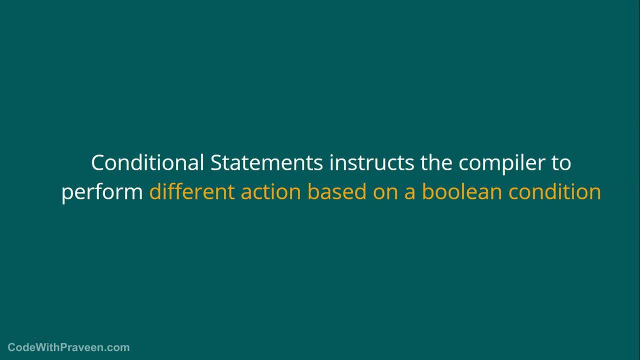 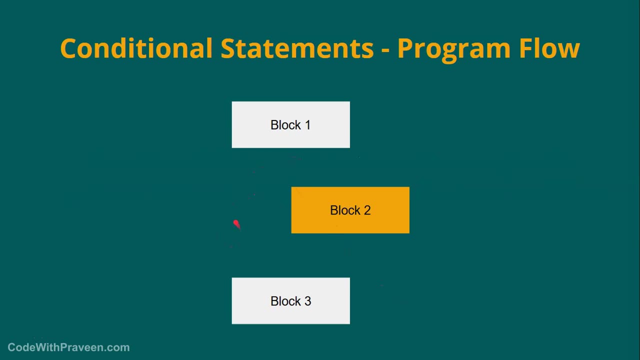 to execute specific action based on certain conditions. Again, let us take these set of examples. Now we again have the block 1, then the block 2 and block 3.. Suppose you want to tell block 2 needs to be executed only if certain condition matches. 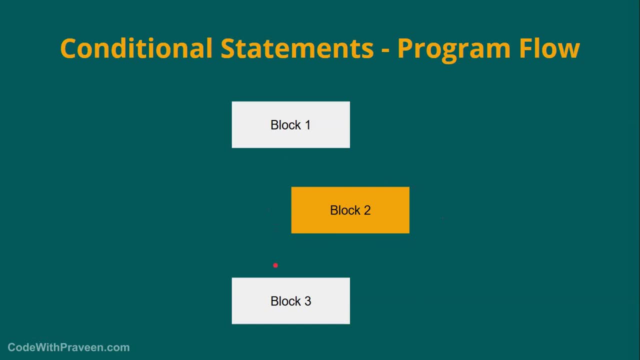 If the condition doesn't match, then it has to execute block 3.. How do you do that? So we use the conditional statements. So our achievement is something like this: So if only the certain specific statement is true, then we execute the block 2.. 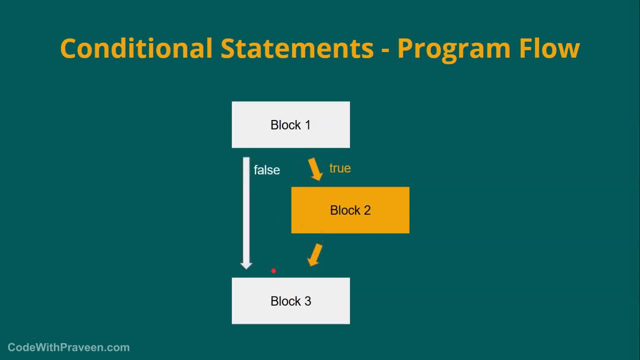 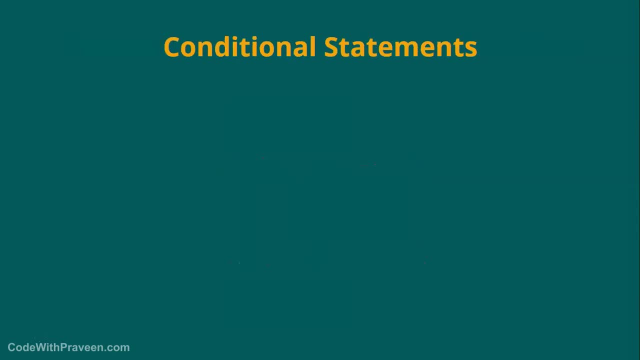 Otherwise, we are going to execute block 3.. So now, how do you implement in a programming language this specific conditional statements? There are many ways we can implement these conditional statements in a typical programming language. Before we move further, I just want to make some points on these statements. 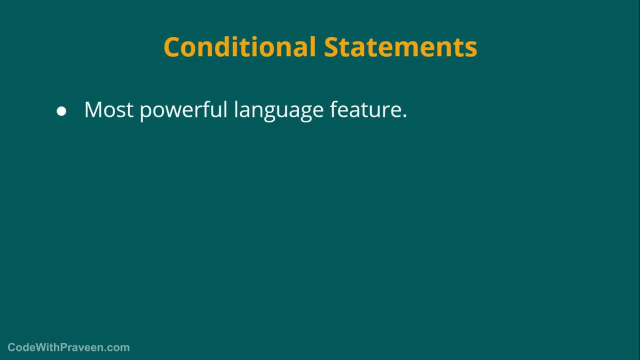 The first is. The first is. The first is: These conditional statements are the most powerful language feature. Personally, I like these conditional statements a lot, The reason being: you can write even the entire function using only these conditional statements, Because they are very simple to use. 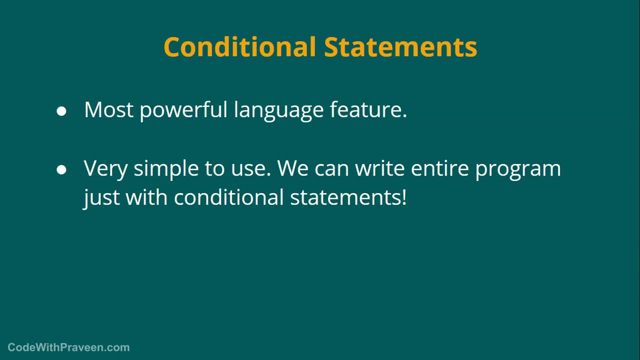 I have seen that there are many code snippets or even the entire functions have been written only using these if conditions. So when you start working in a company, don't get surprised when you see various set of codes which have been written only using these if statements. 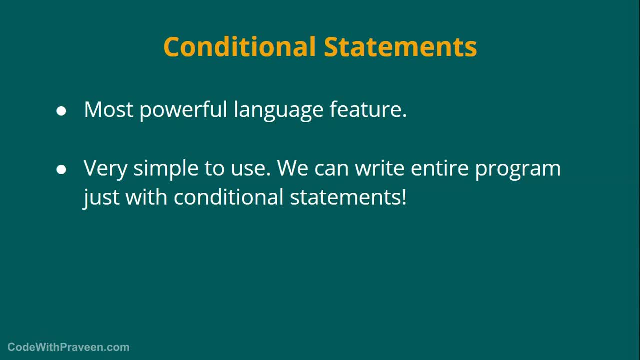 It is possible to write even complex programs using just these conditional statements. Finally, these are also referred to as just conditions, Like you might be hearing. like okay, this is a condition statement or it's just conditions, So they refer to one and the same. 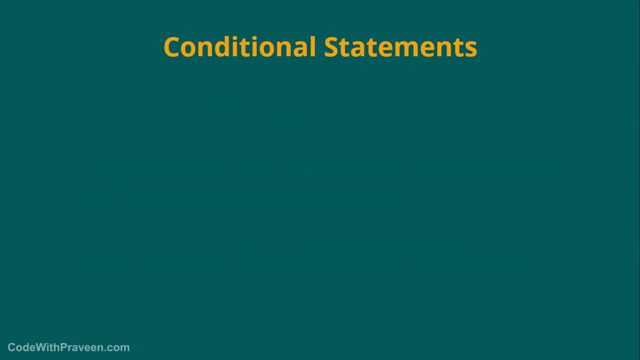 Coming back to the different ways of achieving these conditional logic, we broadly have four different types of conditional statements. They are if, if-else, nested if-else and, finally, switch case. Most of the programming languages supports these types of conditional statements. 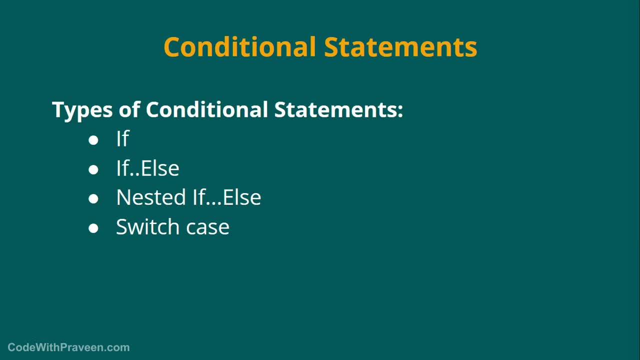 In the next few set of videos. let us cover these different types, one after the other In the next video. let's start with the first type, namely if statement. In this video we will see the first type of conditional statement, namely if statement. 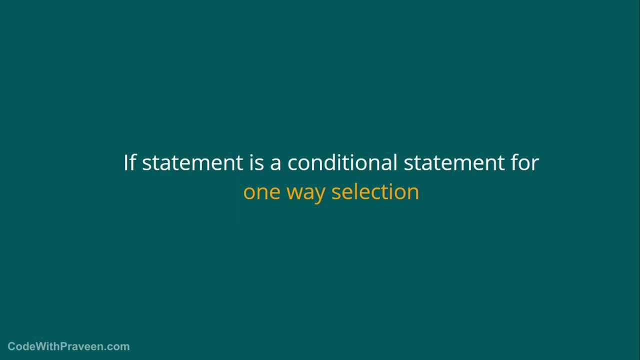 If statement is a conditional statement for one way selection, What it means is that we just have one type of selection methodology to execute one block. So when the program flow executes it will check for a condition. if it satisfies, then it executes a block. otherwise, 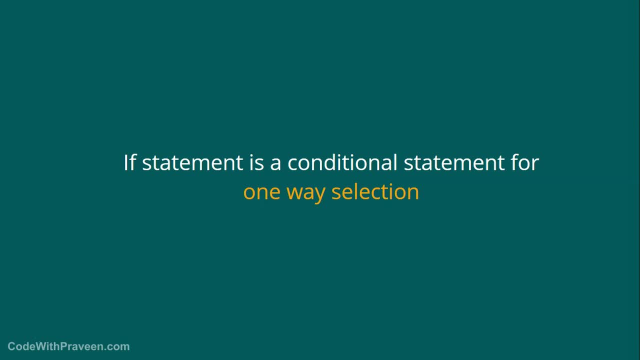 it proceeds. so we literally have just one way of selecting the code snippet. let us see the program flow. in case of the if statement. we here have the if keyword followed by the condition. so what we want to achieve is if this condition executes, and then, if it is true, then execute this set of block. 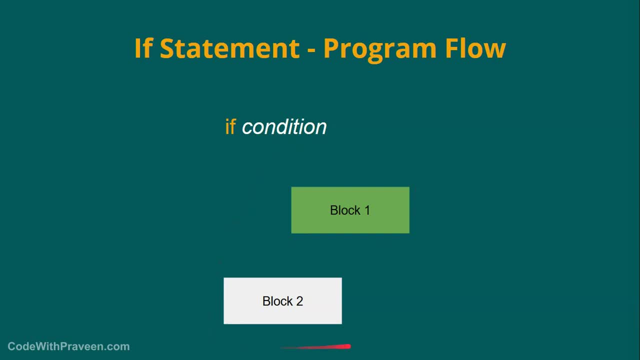 if suppose this condition is false, then you execute only this set of block. so this we want to achieve using say if statement. so the program flow is typically like this. so, as you can see, if condition true, then it executes this block and then this continues with block two. if suppose. 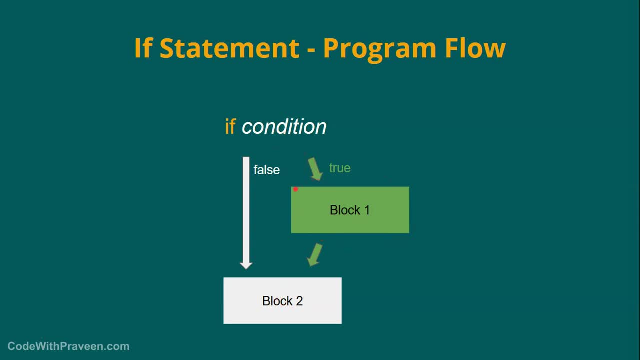 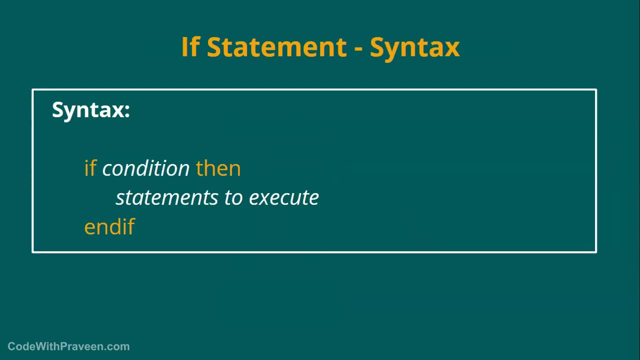 this condition is false, then this is get. this block gets skipped. it directly executes this block two. this is the program flow of a typical if condition. now let us look at the syntax of these if statements. as you can see below, the if statement syntax is quite simple. we have the if keyword, followed by 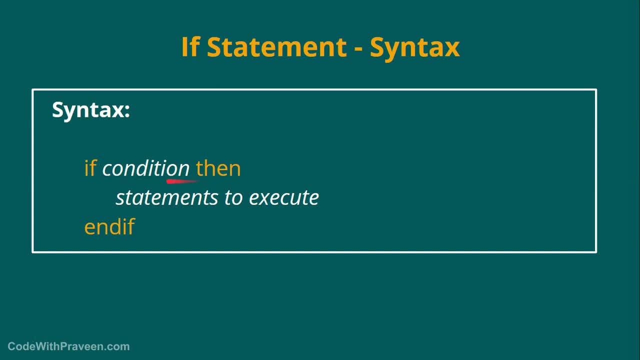 the actual condition, then the then keyword, followed by the statements to execute. finally, we end with end. if so, what happens is if this condition is executed. if it is true, then these statements get executed. otherwise, it comes to the next set of lines, which is over here. let us see couple of examples for these if statements. the first one: 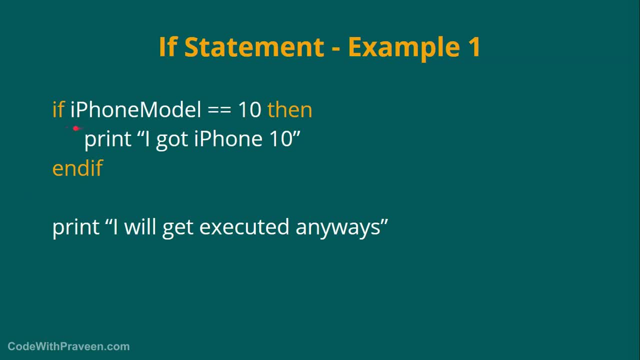 is again our simple iphone model usage. so we want to print the i've got iphone 10 message only if our iphone model is 10.. in other cases we don't print this. so what we do if iphone model equals 10? so in our case this is the condition. 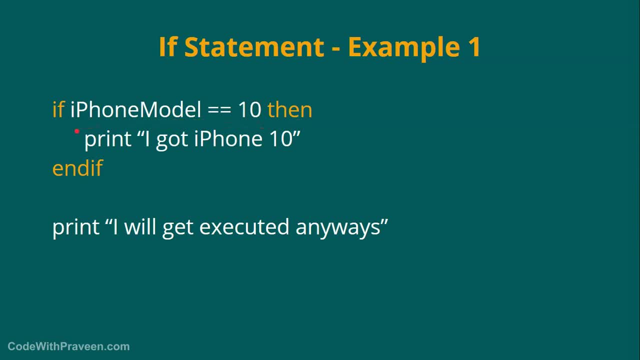 if this condition satisfies, then we print the set of statements. notice that in our example we just have a single line, but in case of actual real world programming you have lot, many lines. so in our case it's very simple: if iphone model equals 10, then we print this, then it ends, then it. 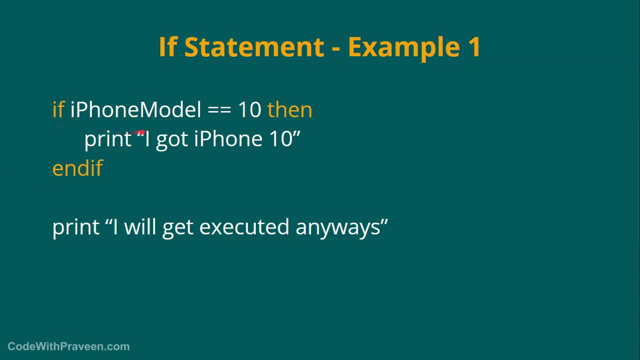 starts executing the next set of statements. suppose, if iphone model is not 10, then what happens is this statement doesn't get printed. this is. this is false. it directly comes over to the next line, which is: print: i will get executed anyways, irrespective of whether it's this condition is. 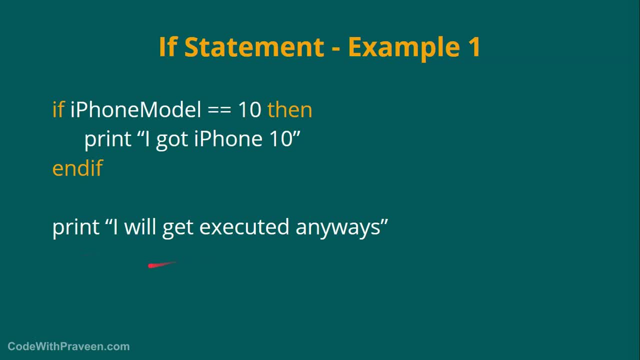 satisfied or not, this statement will get executed because it is outside the if clause. now let us check the set of lines. now let us check the second example, where we try to use two of the conditions. so here we have the if keyword, we have the iphone model equals 10 or iphone model equals 11.. so when the program 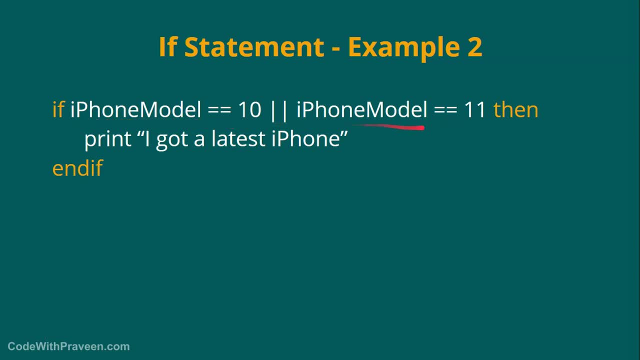 executes, it will check for the phone model to be either 10 or 11.. if either of these two condition is true, then it means this entire statement is considered as true. then it will print. i got a latest iphone. suppose the iphone model is neither 10 nor 11, then 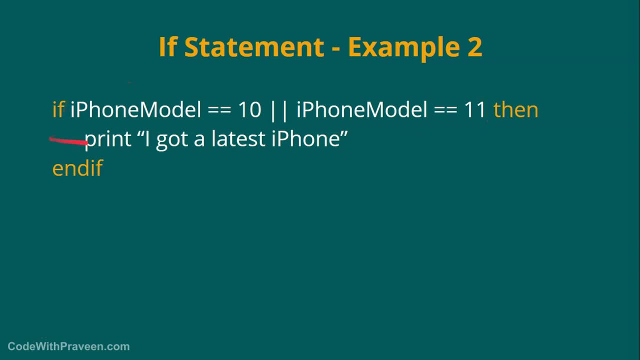 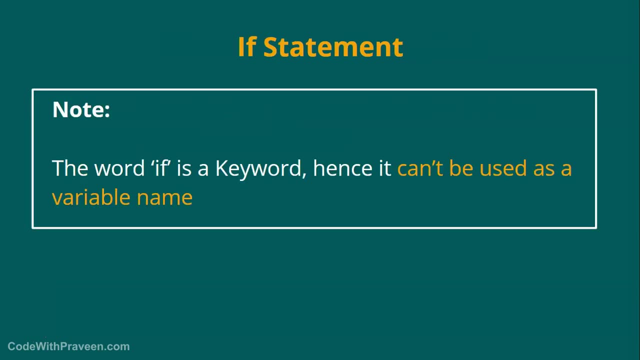 this entire statement evaluates to false, then this statement gets skipped because it's false. then whatever statement is below this, it gets continued execution. note that the word if is a keyword, hence it cannot be used as a variable name. if you remember, keywords are the set of standard variables used by a programming language and you cannot use them in any variable names or. 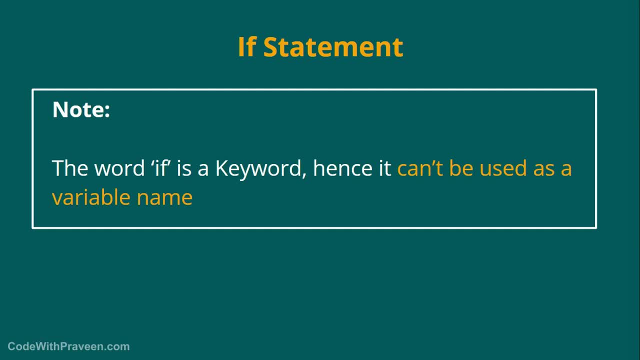 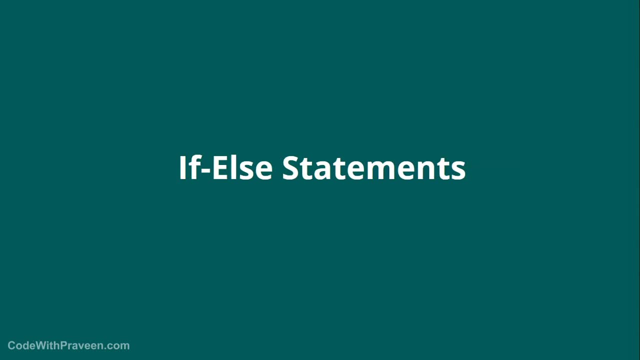 any other constructs. so in our case, if is a keyword, so you cannot use it as a variable name. in the next video we will see the second type of conditional statement, namely if else statements. now let us check: if else statements, if else statements or conditional statements for two. 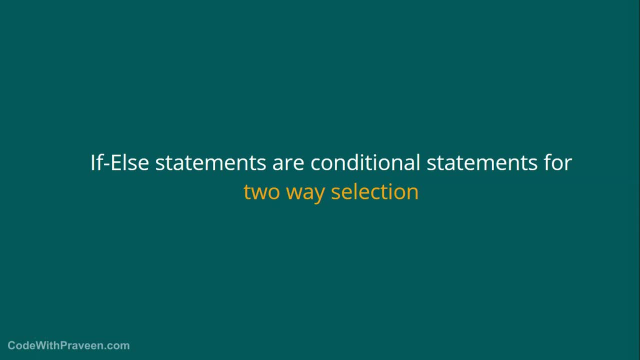 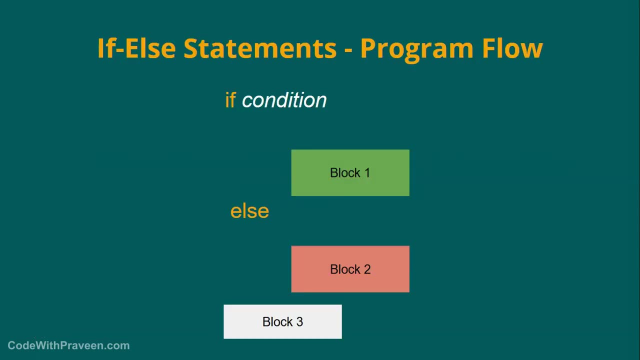 way selection. we saw in the previous video that if statement refers to a one-way selection. now if else refers to a two-way selection. check out this block diagram. let's see what happens in case of a program flow for if else statements. basically, what we are trying to achieve is: 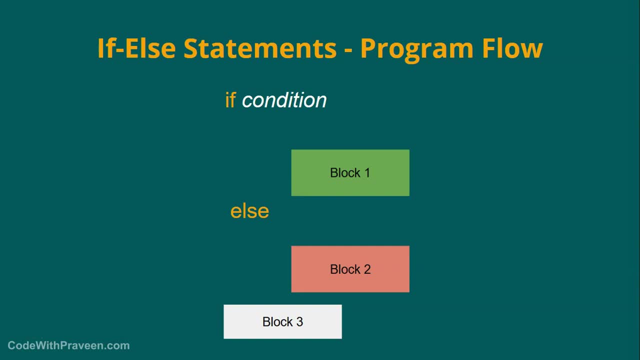 a one block should get executed for when the condition gets succeeded, and the other set of block should get executed if that condition fails. that is the very purpose of these if else statements. the program flow is quite simple. so we have a condition which is being checked. if this condition is true, then this block 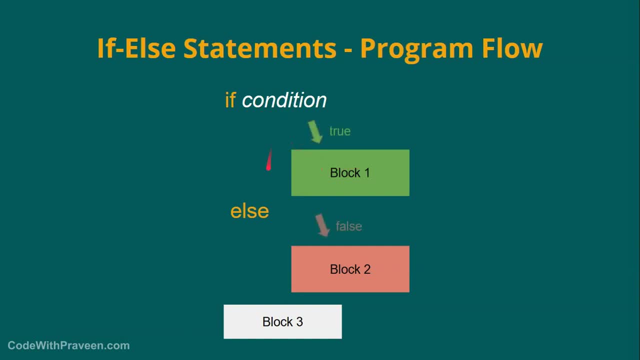 should get executed. if suppose this condition fails, we then want this block to be executed. this is just a simple program flow in case of if else. so, to repeat: if we have a condition which is being evaluated, if it succeeds, which is like true, then this block gets executed. otherwise, if it is false, then this block gets. 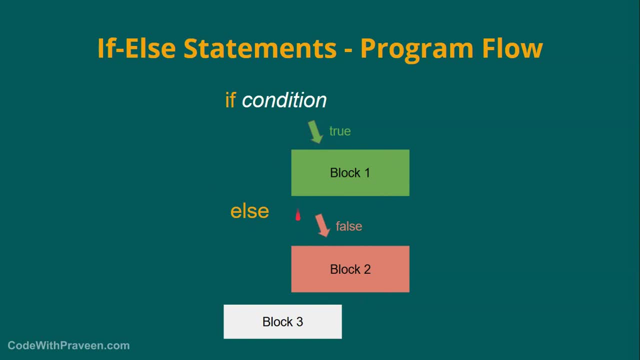 executed, then, irrespective of whether this condition or this block is executed, it continues with execution of all further blocks. as you might have noticed, if either of this block gets executed, the other block doesn't get executed. that is, if this blocks get executed, then it, the control, comes directly to here. in similar fashion, if block 2 gets executed, then it directly comes. 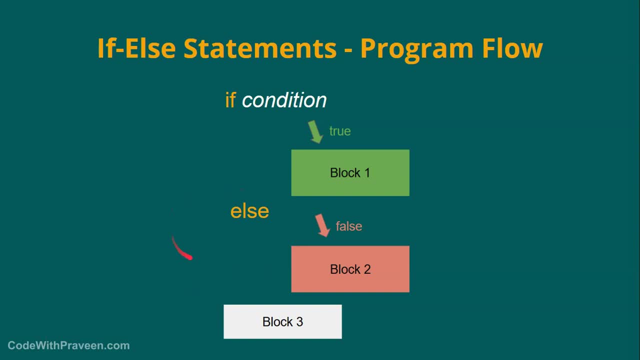 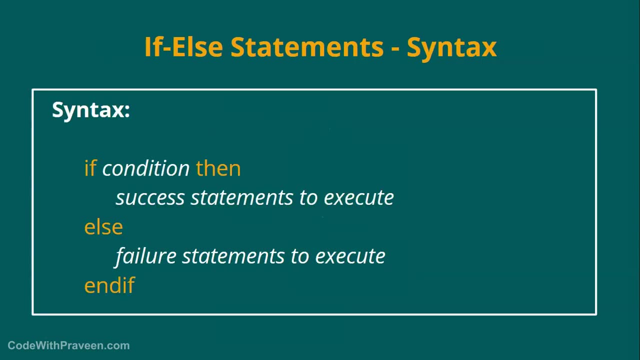 to here. there is no way that block 1 and block 2 get executed at the same time. that is a very fundamental concept of these if else conditions. coming to the syntax of these if else statements, it is very similar to those of if statement, except for the addition of this else clause. 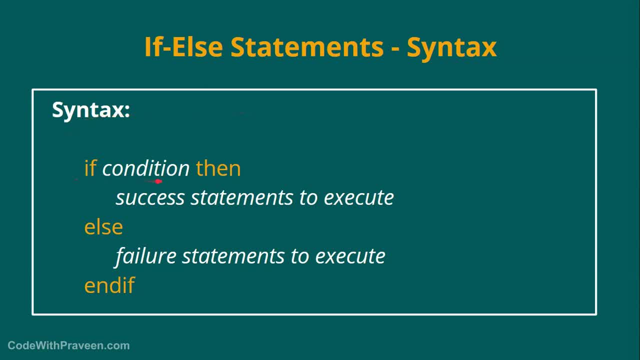 in case of if condition, we saw that if followed by a condition, then we had a then keyword, followed by a set of statements and then end if. the only difference with in if else is this addition of this else clause. so we tell that if this condition succeeds, then these statements, else if we have a keyword. 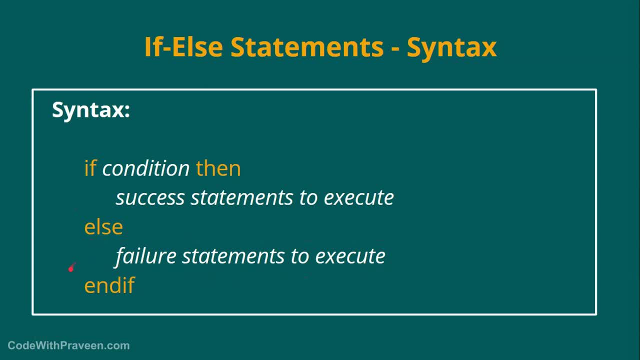 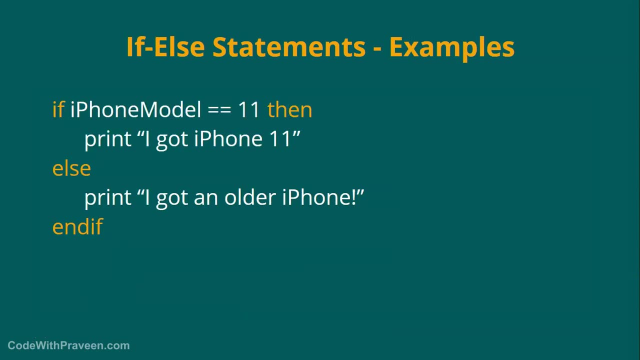 then this set of statements and finally, we end with end. if, irrespective of whether this statements executes or this executes, once it's over, the program will continue with any statements below this end. if keyword, let us go back to our iphone model sample program now here. as you can see, we are trying. 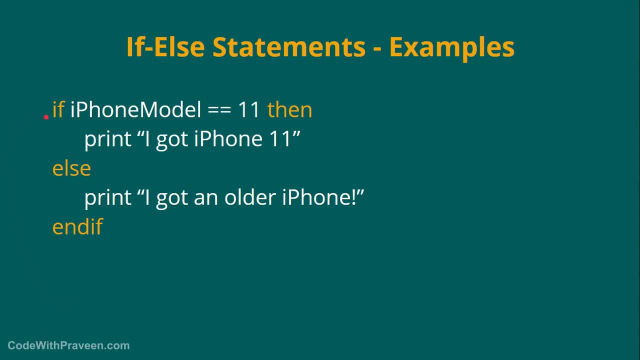 to use the same concept here. as you can see, we are using the same concept here for the same concept. we are using the same concept here for the same concept, here for the same, except that we are using it for if-else statements. we have again the if iPhone. 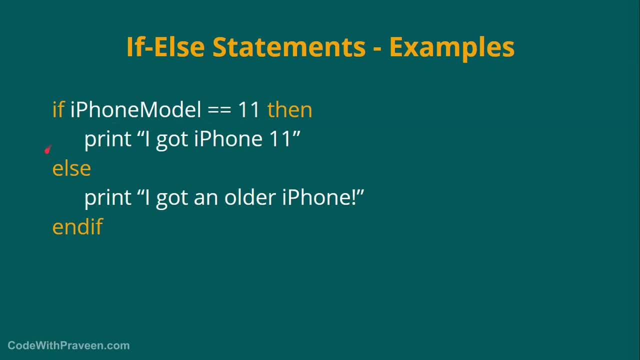 model equals 11, then we are printing the iPhone 11. else in all other cases where iPhone model is not equal to 11, then it prints. I got an older iPhone now. as you can see here, there is no way these two statements can execute at the same time. 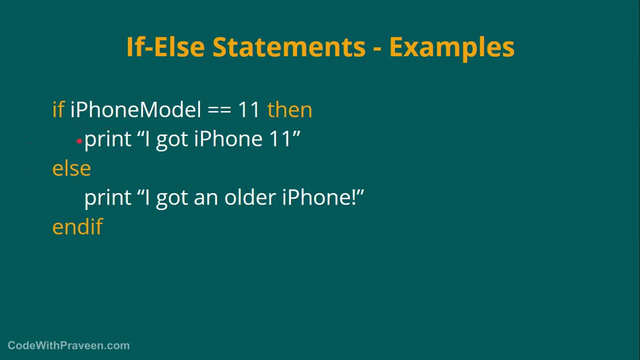 if iPhone model equals 11, then this statement is executed. for any other cases, what this statement is, get executed. there is no way that both statement can execute. now, irrespective of which statement gets executed, once it is completed, any statements below this if, end, if- is going to be get executed. 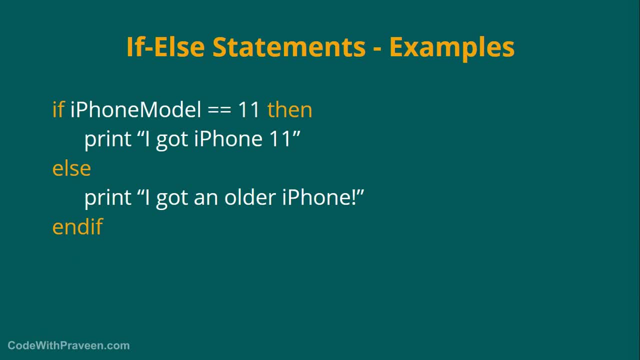 another point I would like to make here is that, just like if statements, in this case of conditions, we can have multiple conditions here, like if iPhone model equals 11 or iPhone model equals 10, then you can say: print: if I got iPhone 11 or 10. so basically this: 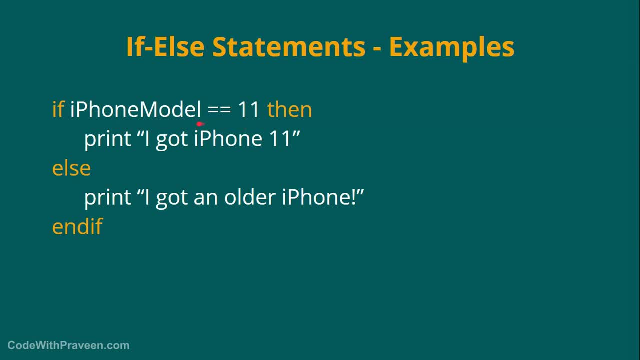 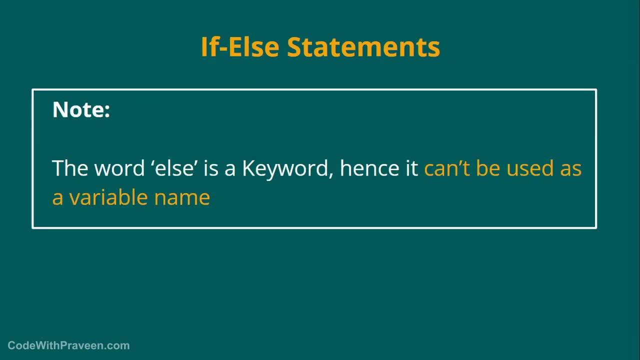 condition need not be a single condition. it can be a multiple if the entire statement should either evaluate to true or false. accordingly, this set of statements is getting executed, as always. the else is a keyword in this case, so we cannot use it as a variable name. so in case of if-else, both if as well as else. 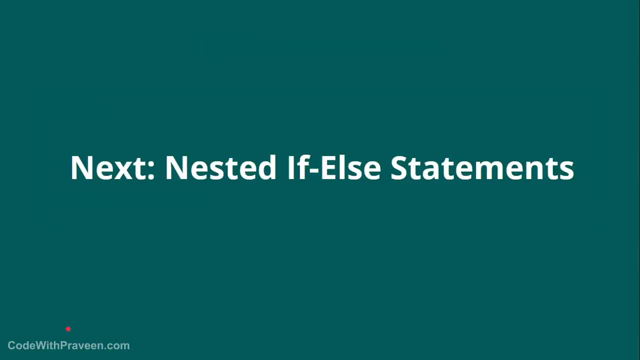 is a keyword, so we cannot use them as variable names. in the next video we will see nested if-else statements. basically, these are just a minor variation of the if or if-else statements which we have seen before. now let us see the third type of conditional statements, namely nested if-else statements. nested. 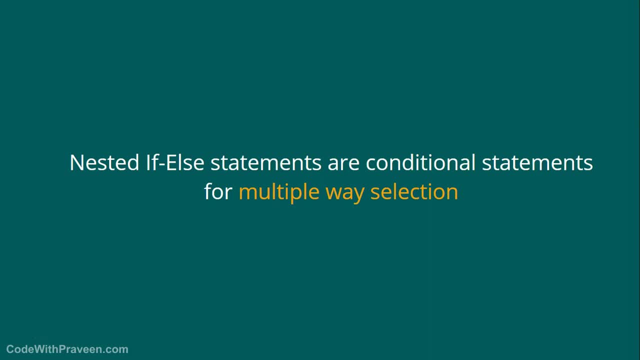 if-else statements or conditional statements for multiple way selection. we have seen before that if is a one way selection, if else is a two way selection. now these nested if-else are used for multiple way. selection is a variant of those if and if else. we try to combine them to form a multiple. 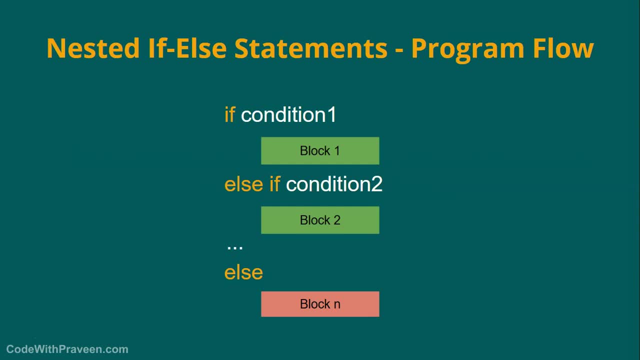 way selection pattern. Let us have a look at the program flow in case of these nested if-else statements. Now, as you can see below, this looks very similar to the if-else conditions which you have seen before. We have the if condition, then the block, then we have say else, then the. 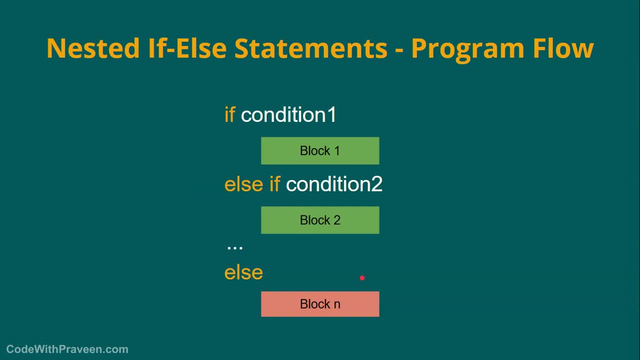 different set of block gets executed Now, the only difference being we have multiple if-else in between. So, as you can see, here we have if, then we followed by another else, if. So basically, what happens is this condition is tried to get true. If it is true, then this block gets executed. 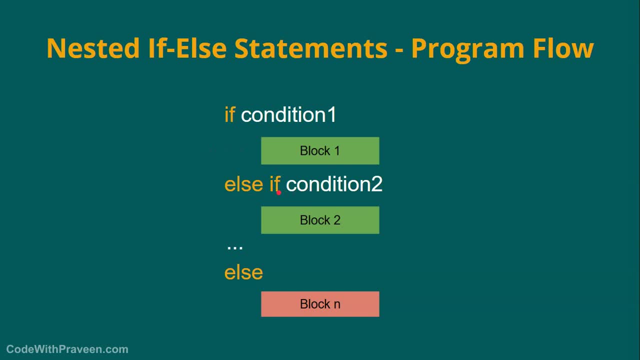 Otherwise it tries to come and execute the second condition. If this condition succeeds, then this block gets executed. Then if suppose we have multiple similar else if conditions, then all these conditions is trying to evaluated. Whichever succeeds, that block gets executed and then the program flow continues after the these nested if-else conditions. Remember that. 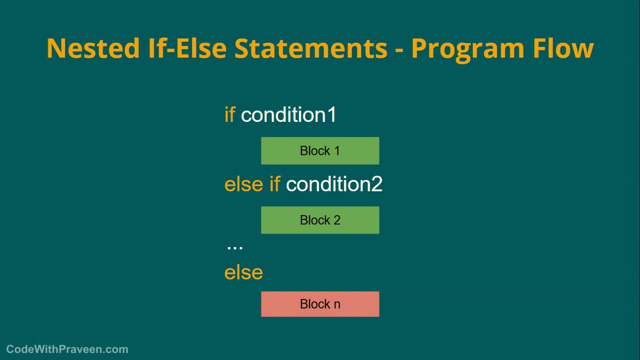 in case of even nested if-else statements, only one block gets executed at a time. So if block one gets executed, then it immediately comes out of all this and the final statement gets executed from here. If this statement is not executed, if neither this and suppose if this statement gets, 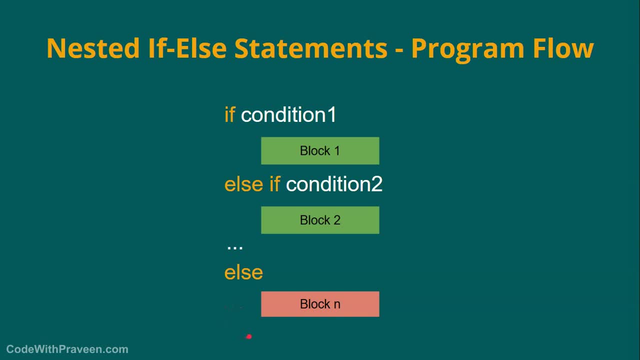 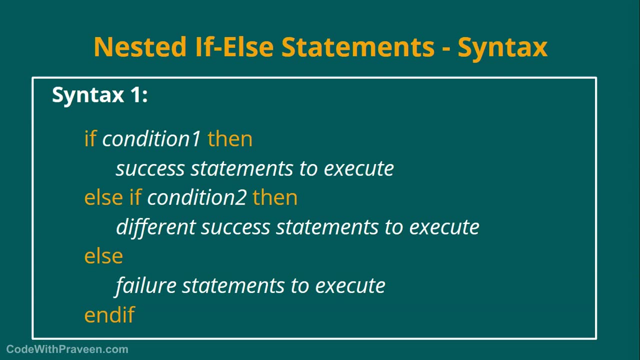 executed as a last resort, then the program execution continues after these if-else conditions. Coming to the summary In the syntax of these nested if-else statements, there are two ways you can achieve this Before we see them. I want to make one point. As you can see in the syntax below, this might 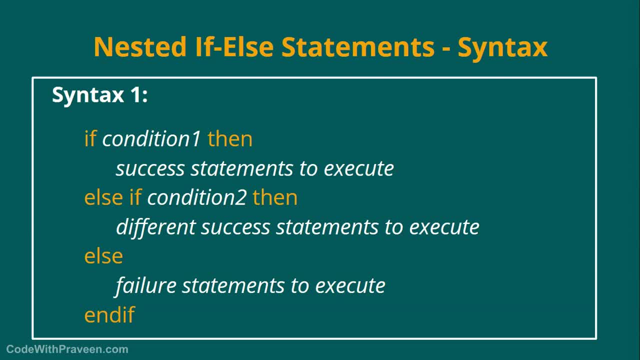 look a bit difficult or a bit complex to understand. If you feel it's being getting difficult, just take your time and then try to understand what this actually statement does, Because I agree that these nested if-else can become tricky and become complex over a period. 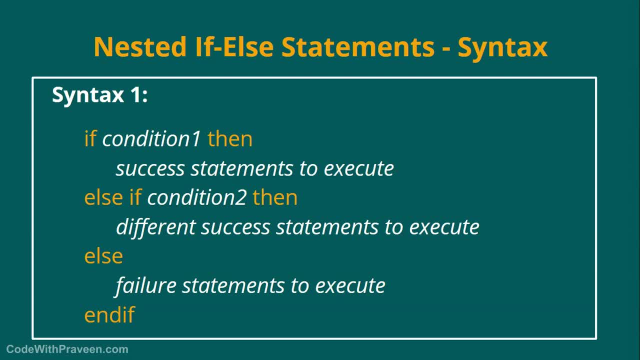 of time, But just spend some time, then you will be able to understand them. In the first syntax we have multiple if conditions, one after the other. So as you can see here, we have first if condition, then we have another if condition, then, like that, you can keep repeating n number of times. 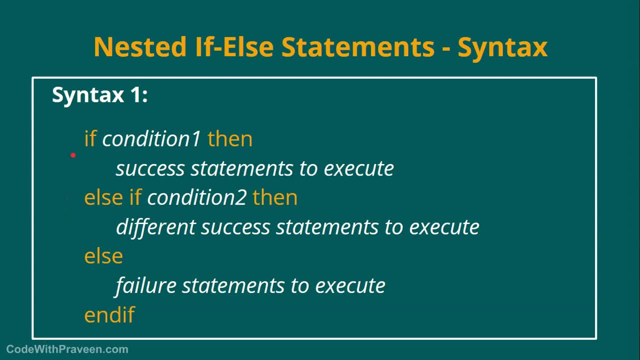 So this is the first way of achieving the nested if-else. Basically, you have multiple if conditions, one after the other. So in this first syntax we have: if condition one, then these statements executed Else, if this condition two succeeds, then this statement Like this you can have for: 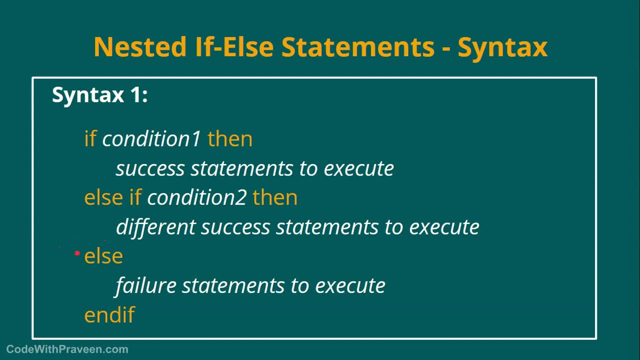 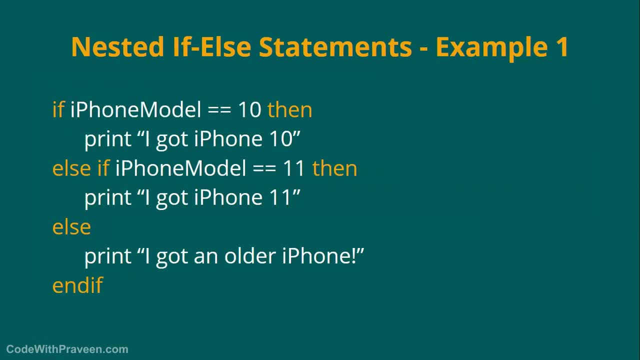 n number of conditions, then ending in if with else. So as you can see, here we have multiple if conditions. That is the first syntax of these nested if else statements. As always, example is a lot better than the theoretical part. So now if 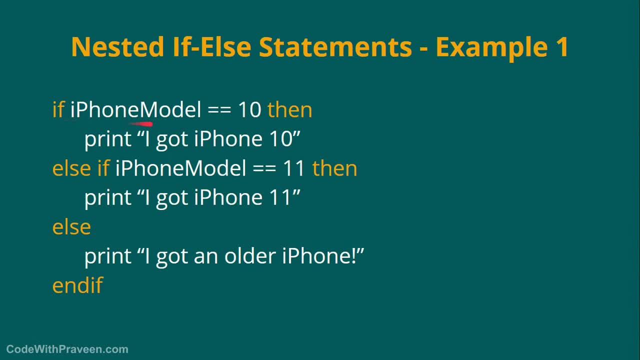 you can see, here we are again using the iPhone model example. Now you see how clean it is. now We have: iPhone model equals 10,, then print 10.. If the iPhone model equals 11,, then print 11.. Like, you can keep repeating it. Like say, if your iPhone model equals 8,, then print 8.. If iPhone 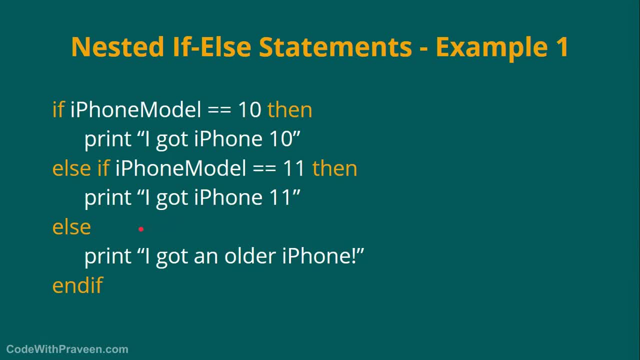 model equals 7, you can print 7.. You can keep going: multiple if conditions. So, as you can see, we are stacking each if conditions one after the other. We are nesting one among the other. That's why it is called as say, nested if else statements. So in our example, the iPhone model is a variable. 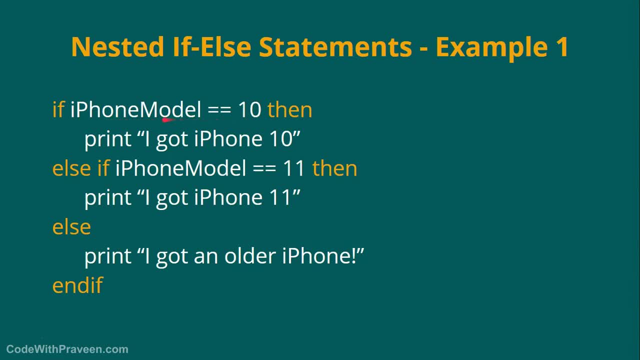 name It is being used and checked against different values. It executes one after the condition until the condition matches. Once the condition matches, then it will print the statements. Now let's come back to the final end. if And whichever statement is below, this is going to get executed. 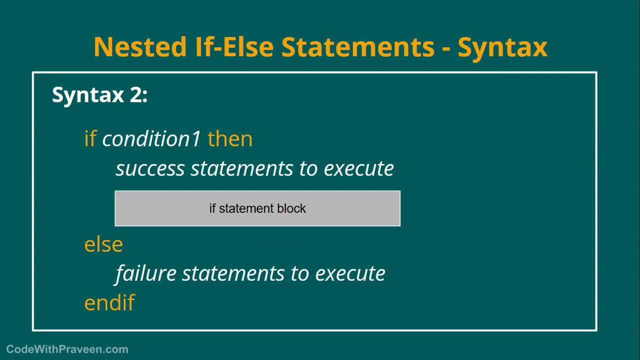 Now this is the second syntax of using these nested if else. Now, as you can see, here we have a simple if else, like say, if condition one, then set of statements to execute, And then we have else, then set of statements to execute. Now how we come back to this nested type is we introduce another if else. 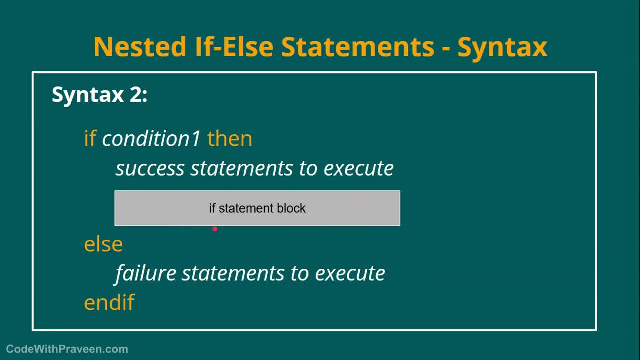 between these if statement, So if condition, then these set of statements get executed. While it executes these statement, we have another if statement or if else statement between this And then we have the else clause for the other set of statements. I understand it's a bit difficult here, but just try to grasp the concept. 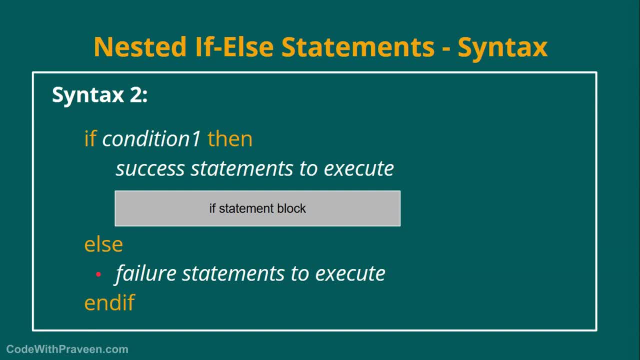 Basically we are nesting multiple if else conditions inside another, if conditions, As always, these nesting can go any level of deeper, Like say you can have if condition, then another, if else condition inside this, then you can have another if else condition inside this. There are basically no limit on that. 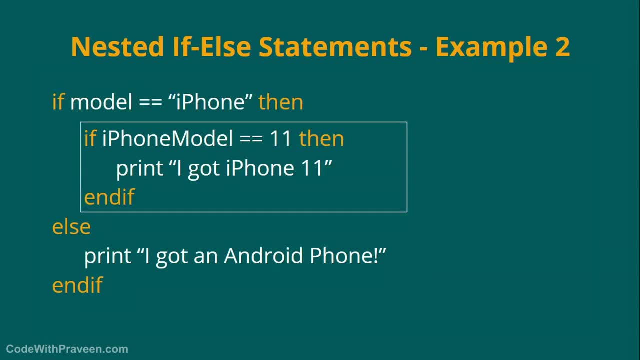 This is the general syntax of these if else statements. Check out the second example for nested if else statements. For now you just skip this block snippet. We'll come back to this shortly. So first we have the if model equals iPhone, then this block gets executed. 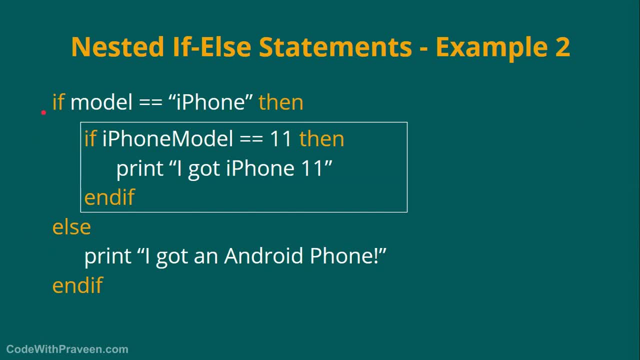 Otherwise, this block gets executed. Now, so far, this is a very simple if else condition, If else statements. So what, basically, we are going to do now is if this statement gets executed, instead of a simple set of statements, we have another if condition here. 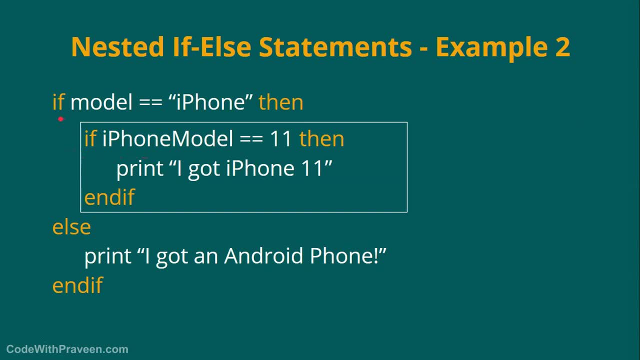 So we are nesting one if inside another if statement. That's why we call it as nested. if, Of course, you can have these if statements any level below, Like iPhone model equals 11,, then instead of printing you can even have other condition, like if iPhone price equals 1000 or something like that. 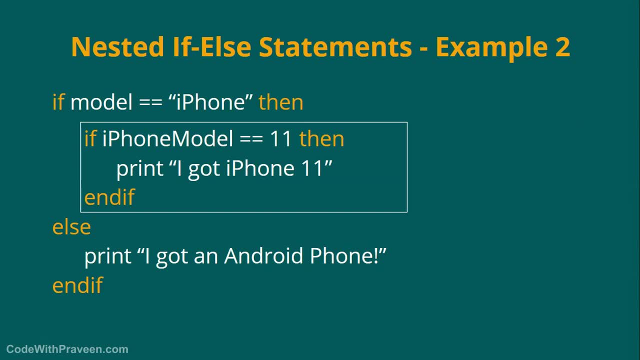 So the nesting of these if-else statements is endless. A quick note on this nested if-else statement is that don't make it too complicated. Don't try to have multiple nested if-else statements just because the programming language allows it. You have to be careful with having the multiple levels of these if-else statements. 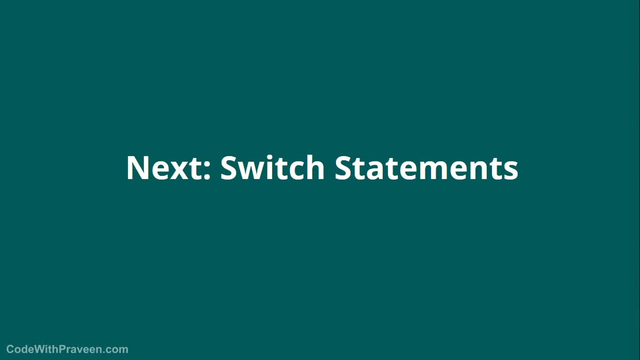 In the next video we will see the final type of conditional statements, namely switch statements. This is basically a variation of these nested if-else statements, but in a lot easier way to maintain a lot more of these if-else statements. So the nesting of these if-else statements is endless. 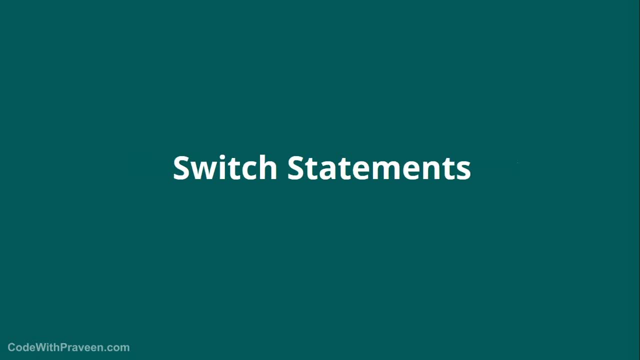 So the nesting of these if-else statements is endless, As well as a better readability. Now let us see the final type of conditional statement, namely switch statements. Switch statements are conditional statements for multiple way selection. Again, the definition looks very similar to nested if-else. 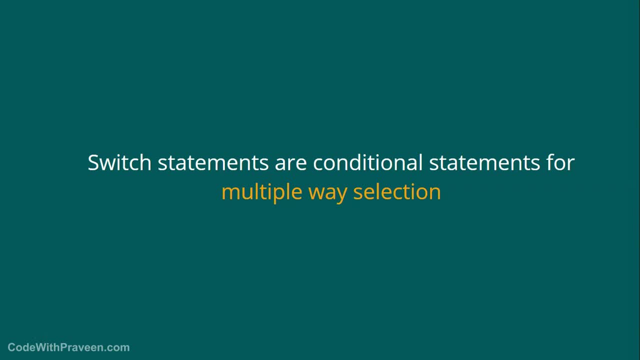 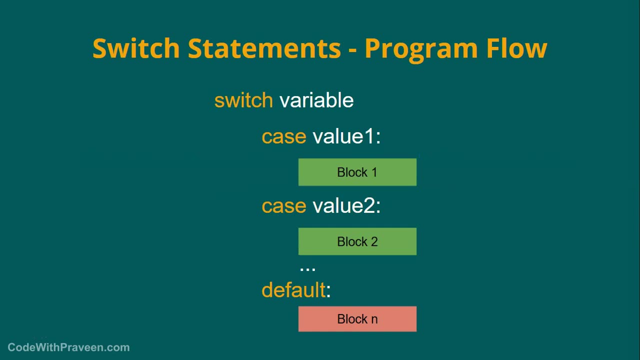 In fact, these both are very close to each other, except for the change in their representation or syntax. Let us check the program flow in case of these switch statements. As you can see below, it is a bit different from all those if-else conditions. 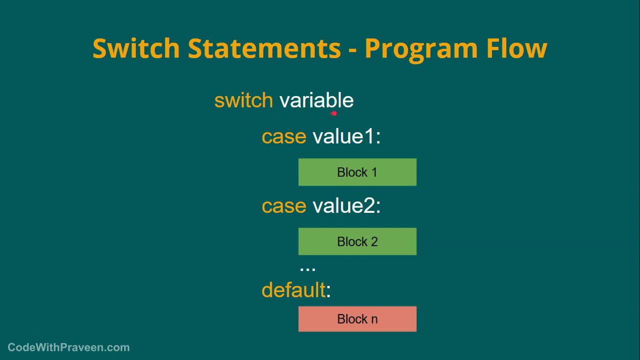 We have the switch keyword followed by a variable name, Then we have a case keyword followed by a value, Then we have these blocks. So, as you can see, we have multiple blocks and finally a default block. What the flow actually tells is that we try to check the value of this variable. 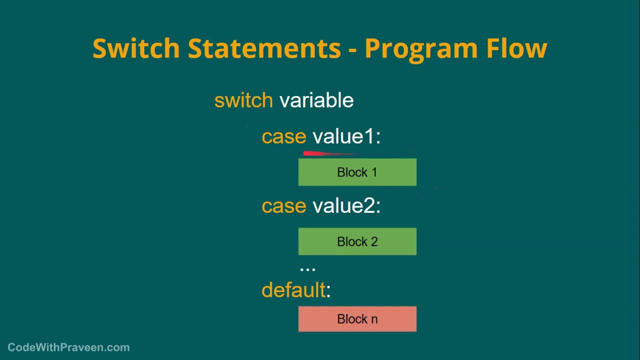 And, depending on the value, we try to execute a set of blocks. Now it is a bit different from the way we have been seeing for these nested if-else or if-else conditions. A very big advantage of this switch statement is that it is very readable. 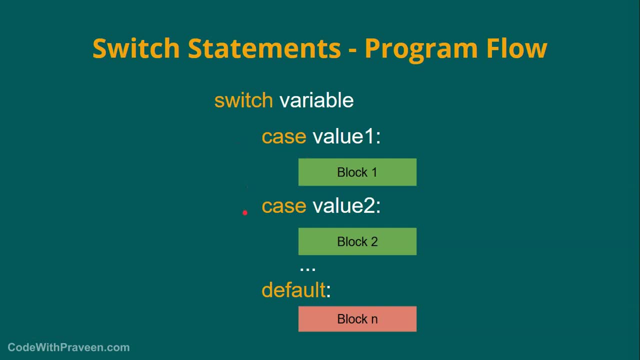 As you can see, it is very easy. You can see this is first block, this is second block and this third block and say final block. We saw that in case of nested if-else it can really get complicated, But switch case statements are a bit easier to read and easier to maintain as well. 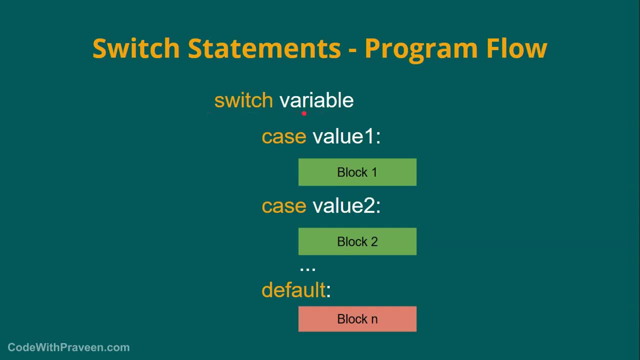 So how the program flow is like that variable name is trying to execute. If this value gets satisfied, then this block gets executed, And then it is a bit more easy to read. And then it comes to the next statement, which is after the switch statement. 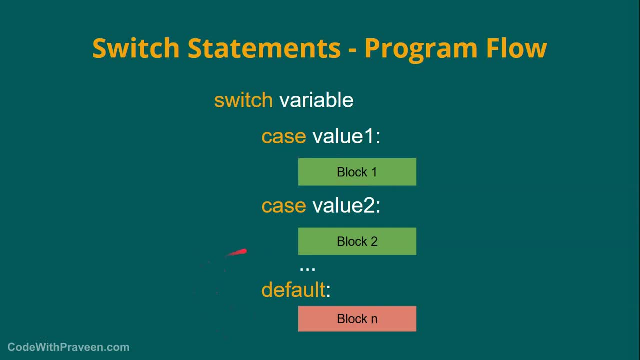 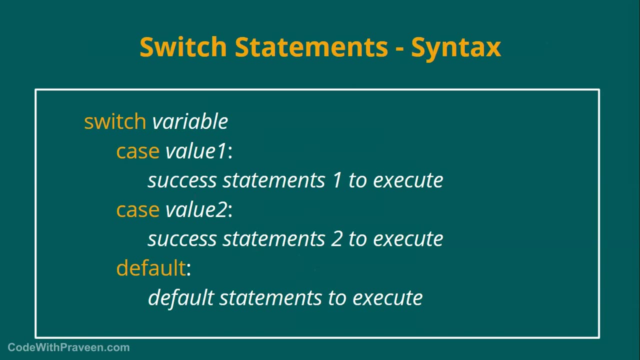 As always, this set of blocks gets skipped when one of the conditions succeeds. That is how the switch statements works. If you have understood the program flow of the switch statements, then the syntax becomes very obvious. So we have the switch keyword followed by the variable name. 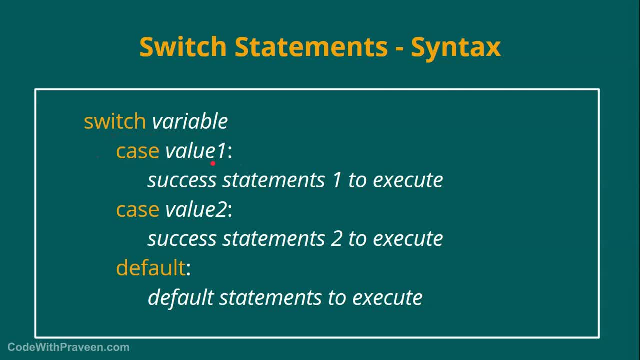 Then we have the case keywords, followed by the actual value. Then we have the statements to execute. Now this can execute any number of times, Depending on the value which you want to check. So in this case, say, valid up to value 2 is being checked. 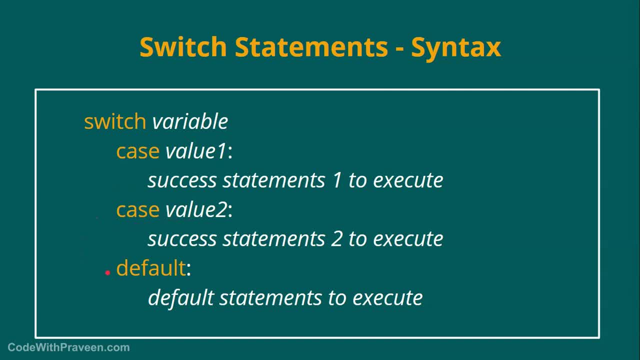 And we have the default case. Now, what is this default? What it means is that when you are checking for this variable name, if none of these cases get satisfied, then this statement gets executed. As you can relate, this is equivalent to the else clause in case of if-else statements. 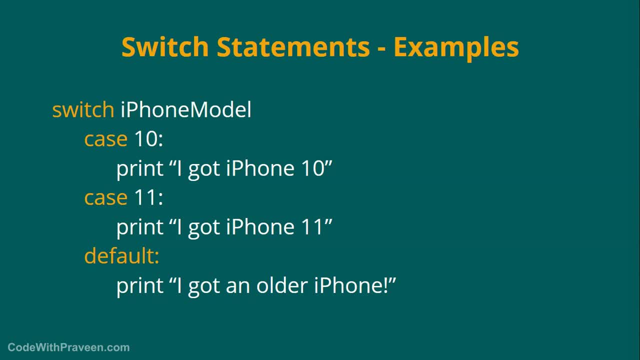 Now, going back to our iPhone model examples, let's see how it is represented in case of switch statements. Here we have the iPhone model as a variable name. Then we have multiple case statements with the value we are checking. So in case of value 10, we print iPhone 10.. 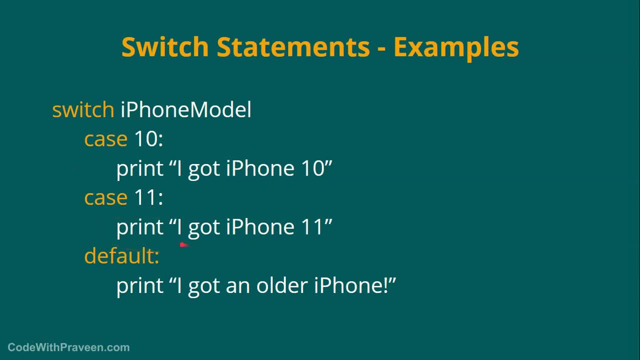 In case of value 11,, we print iPhone 11 and so on. Suppose, if none of these conditions get satisfied, then we have the default clause, which prints: I've got an older iPhone Now. as you can see here, this is very similar to what we saw in case of nested if-else, except that it's a lot more easy to understand as well as a lot more easier to manage. 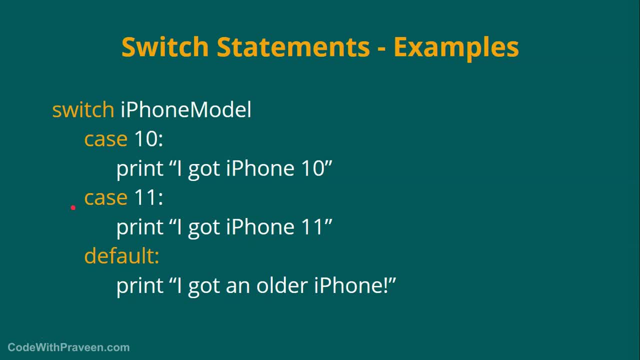 Meaning that tomorrow, if the new iPhone model gets released, then you just add one more case, say case 12, print: I got iPhone 12,. same way if we have, say, 13,, 14,, 15 and so on, it's easy to maintain as well as it's easy to remember and easy to maintain at the same time.